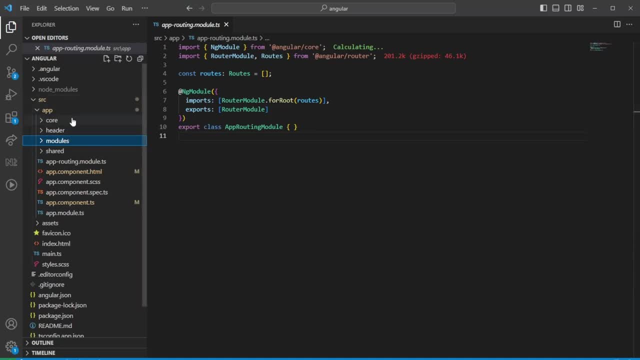 modules and let's break them down. so the core- the core folder in this case- would essentially contain the code that's shared across the entire application, so it would be application level stuff. so this would mean, for instance, the header component is: is used within the whole application. it would be a perfect thing. 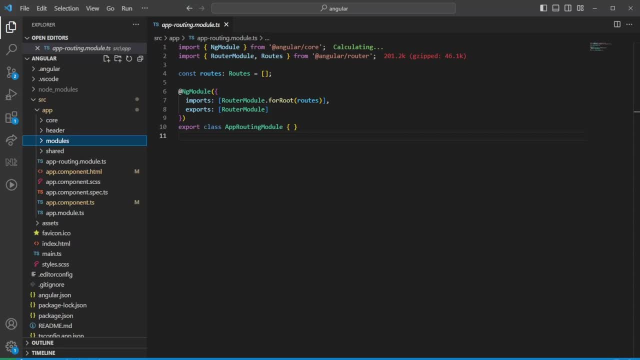 to place within the core utilities here. so in this case, what I would do is create another folder here, which is components. I would drag the header component into the components and also keep in mind that you, you usually want to have a module as well, so we'll generate a module ng. 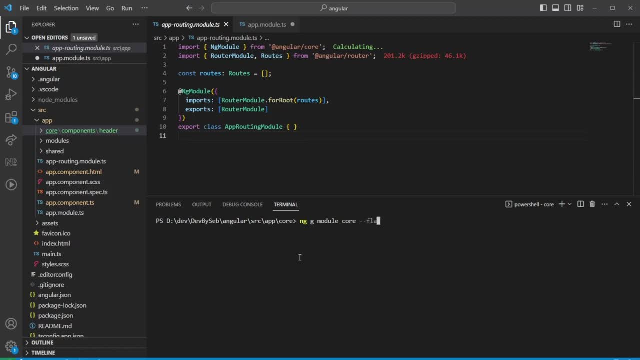 generate module- let's call it core- and then we'll create flat because we already have the. we already have the folder here, so there's no need to to generate the folders. so once this is done, you will see it will generate a core module within this folder here and we'll have the components here. so 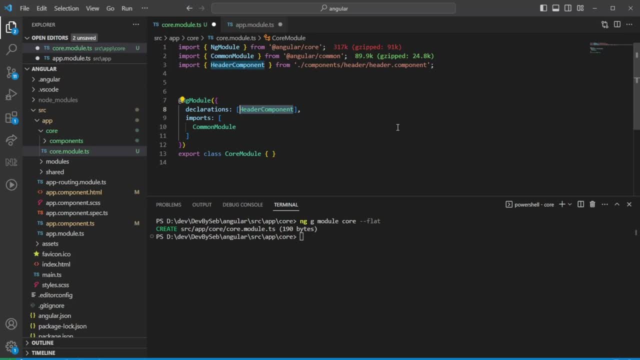 obviously you should declare the header component and then you should create the header component here, and it also needs to be exported here, because this is what we want to use from the app component TS file. so what we need to do now is essentially remove the components from here. try to keep the app module as clean. 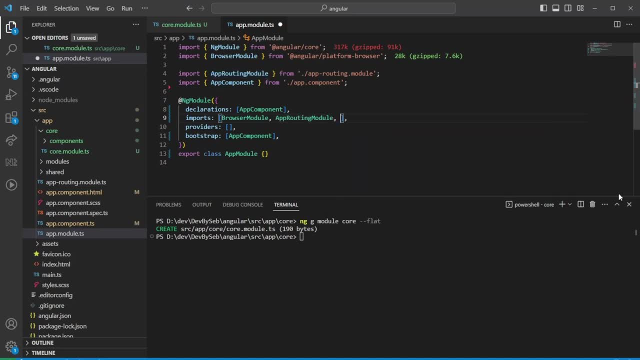 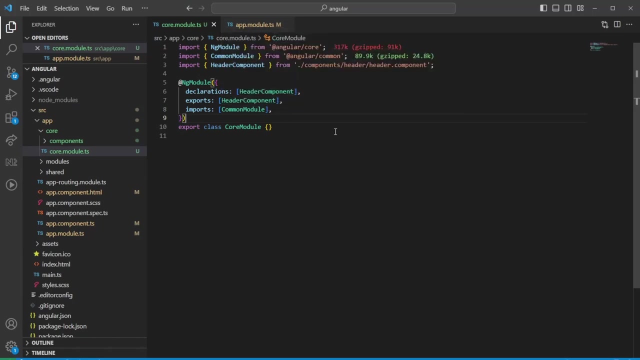 as possible. try not to use too much stuff. I this is just a tip for me, because it will be so much easier for you in the long run when you keep it quite basic and simple. simplicity is key when we are talking about Enterprise applications, because we're going to have to teach and educate new developers. 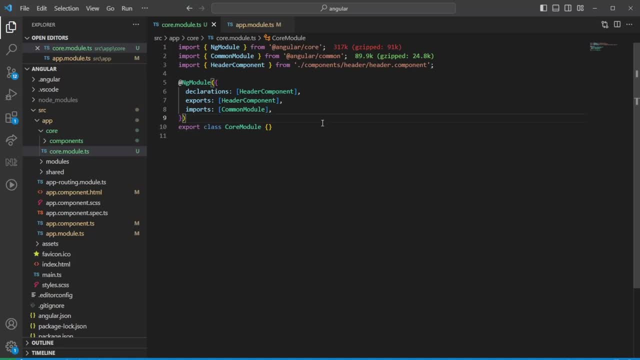 coming into the project at the same time. we need to maintain a structure which follows the best practices. so, all right, we have the core module and we are importing everything from the core stuff into the core module. so here we could have. it could be guards, authentication guards, it could be other guards that we 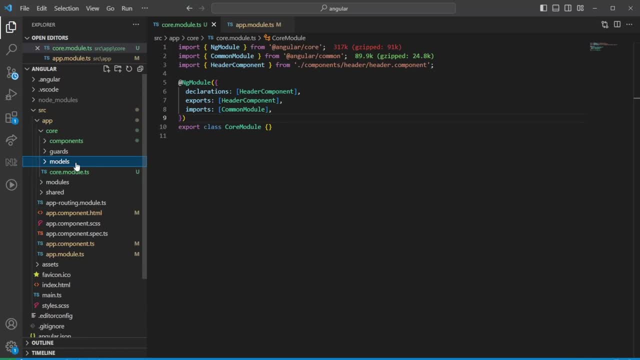 have. so it could be core models. I would say these core models would be just related to whatever you have within the core, so it would not be something that you potentially have in the shared folder. so just try to keep it simple, try to keep everything here just related to itself. 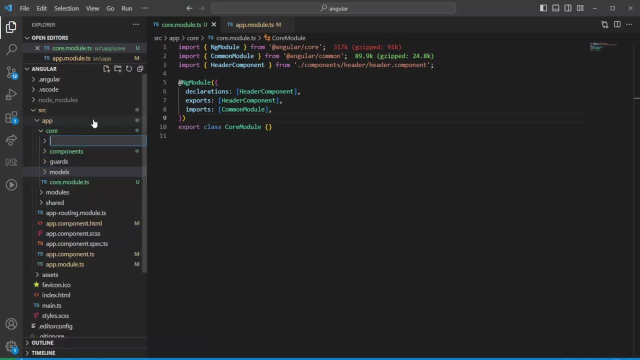 so that we easily can break out stuff and so on. and of course we have services. this could be the language services that we have, or any extensions. we could also have utils or constants here. so constants- really anything related to the general structure- would be in in here. so 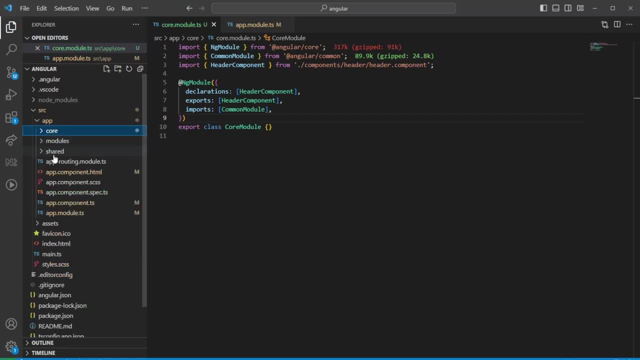 all code that is shared across the entire application. so you might think now, what's the difference between the core and the shared? so this shared folder could be thought of as different stuff that's shared amongst the modules that we have. so it could be for a, for instance, it could be the UI component library. so UI in this case it. 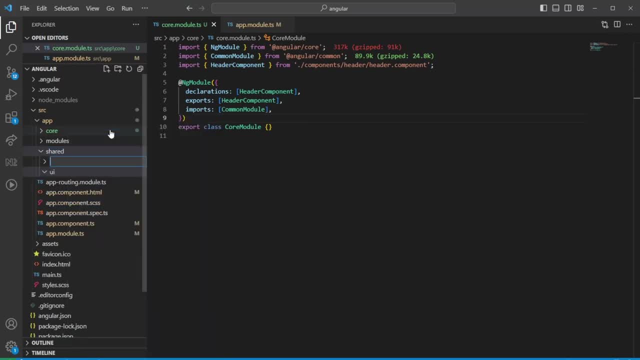 could be. uh, it could be. it could be components, it could be utils. maybe you have utility functions that you're having here, which is essentially needed for the modules, and, yeah, this is like a common pattern that you could have. so think of the shared as stuff, that's. 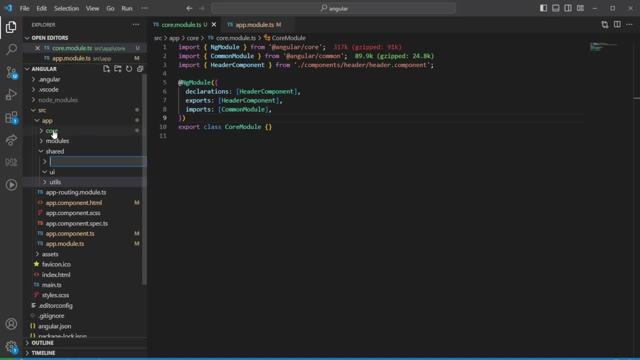 being shared amongst multiple modules. meanwhile, the core is something that that is generalized or used amongst the whole application that you have. try to not have any pair dependencies within the modules. so if you have one module, I'm going to talk to you shortly about what the module is and what you should place within the 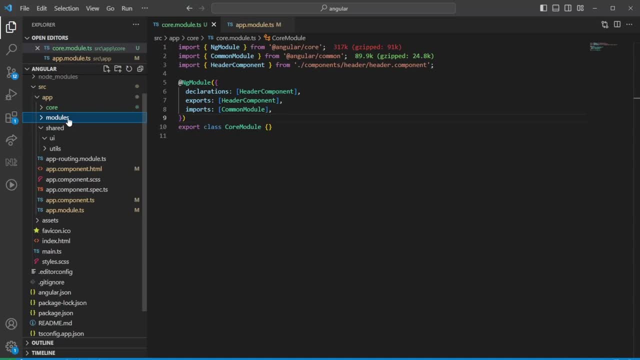 module. some people call it, as I mentioned before, features. usually I tend to call them modules. so what we haven't done here is we haven't created the, the module for the generate module for the shared map. also keep in mind. this is a big mistake many people do. they import everything within this. 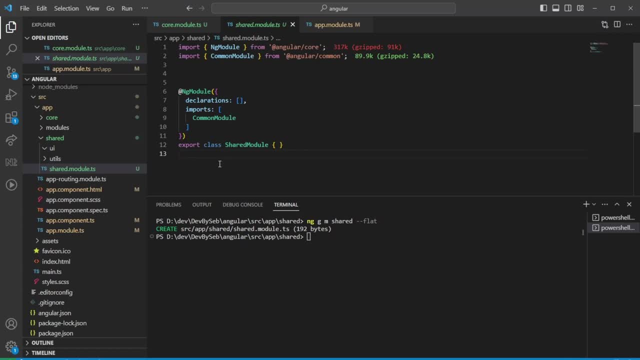 shared module. this is something you definitely don't want to do, because you don't want to use it to do. what we would, or should do essentially, is to utilize tree shake ability in this case, for instance, if we were having a UI component. um, so I will generate a module there, for, let's say, we have 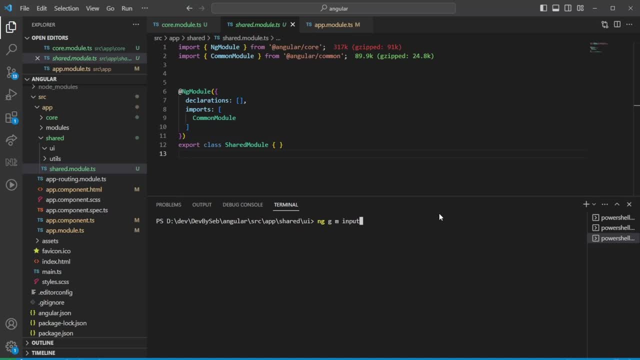 an input module. uh, we'll generate a module called input. in this case I'm not going to use the flat flag, because I wanted to generate a folder and then place it within the folder, so input, input module. so now I would just go ahead and generate a component as well, just to visualize how this would. 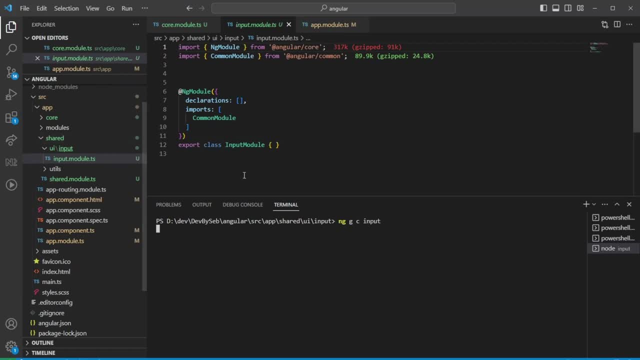 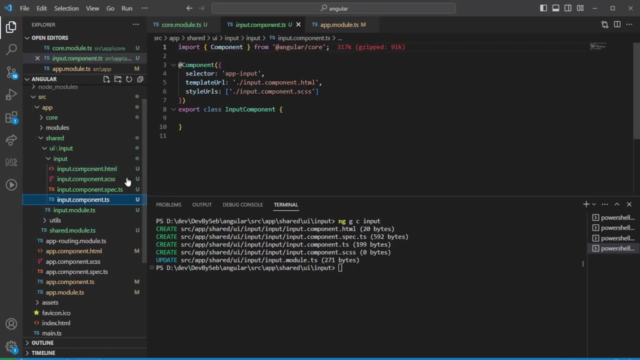 work so good and regenerate component, input component, and now we would have the input component here within the input module, and now we can import- sorry, it should be the declarations we should export, so exporting the component. so what will this do? if we essentially export the input module from the shared module, it would mean that we would 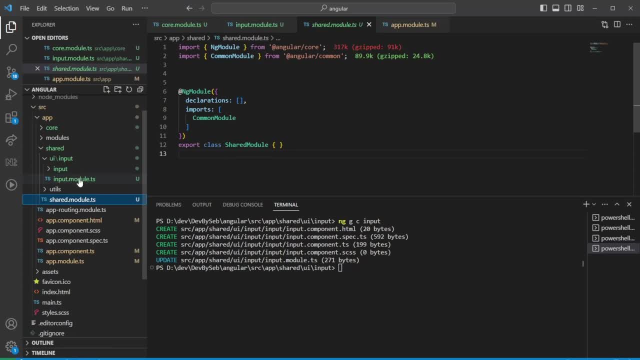 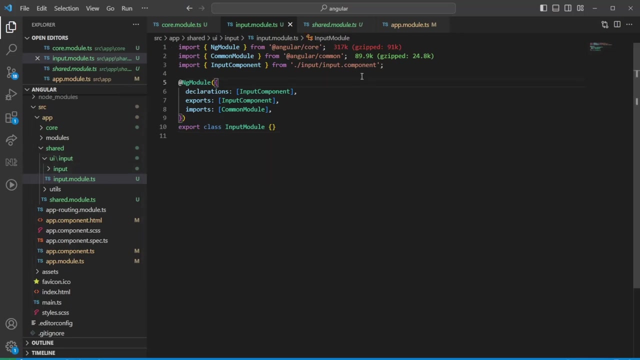 have to import all of the different input components in all different places, and this is something we do not want to do. so we can do this by having a true shake ability within our component in this way. so one thing you could do if you, if you don't want to have this annoying import statements. 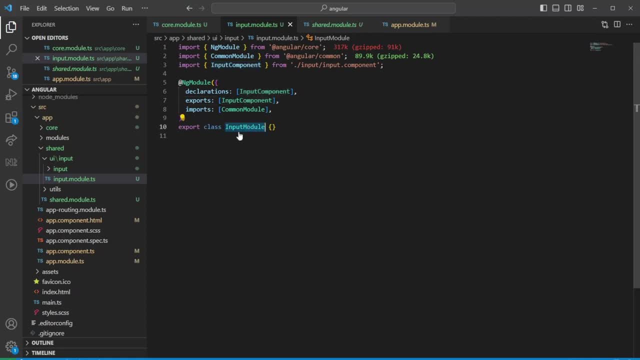 from the code is to essentially combine it with some ts-config that you could use. so I will get to that quite shortly. as long as we have spoken about it, bit more about the shared module. so yeah, so if, in order to use this input module, you would have. 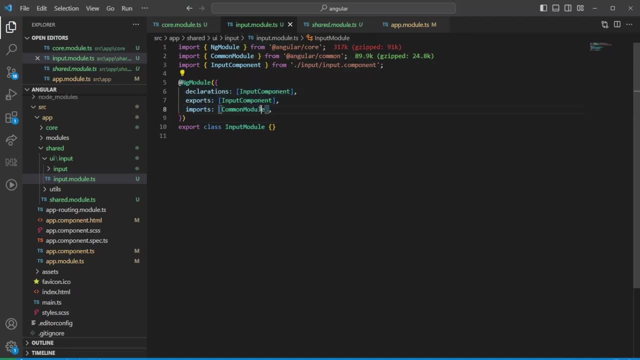 to import the input module, which means that we in this set will only import whatever comes from here, so we will not have to import all of the different stuff that would exist within the shared module, and this is something i would recommend doing. i've seen multiple times where you have a shared 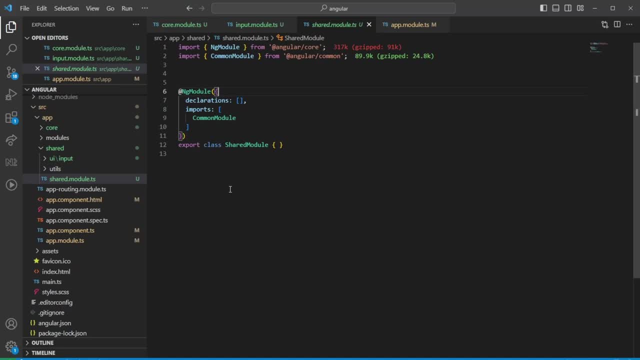 module, which is like 100 things that you're important exporting. i think this is something you definitely should avoid, something that i would mention to be shared. it might be maybe, if you have translations- you have you're exporting the translation module for a child that you want. 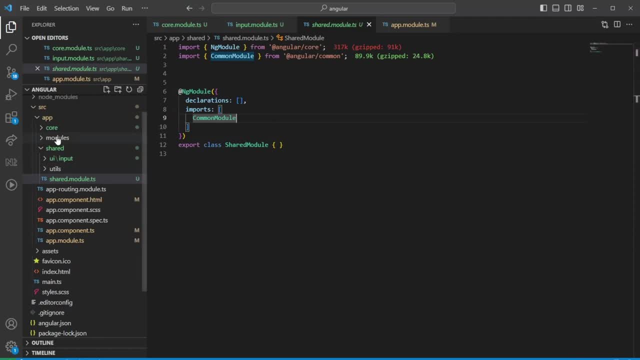 to utilize in the different modules. so you would have to define within the app module you would define translate module for root, you would set up the how the logic should be and here you could essentially just import and export a translate module for root. so something that would be. 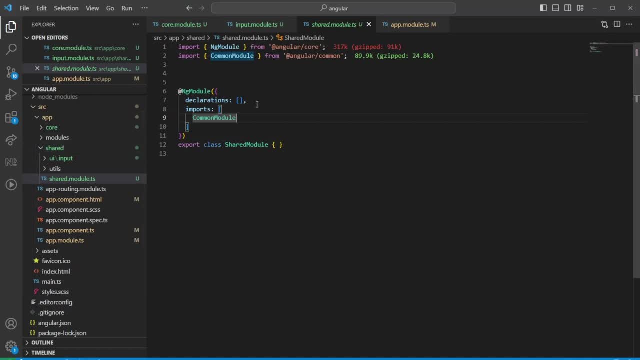 widely used within every module that we have. if you would have translation per se, all right. so now we, once we are breaking down the shared folder and of course, here we could have shared services. we could have shared- yeah, you name it, it could be shared pipes, it could be shared directives, that we have, anything that would be shared. 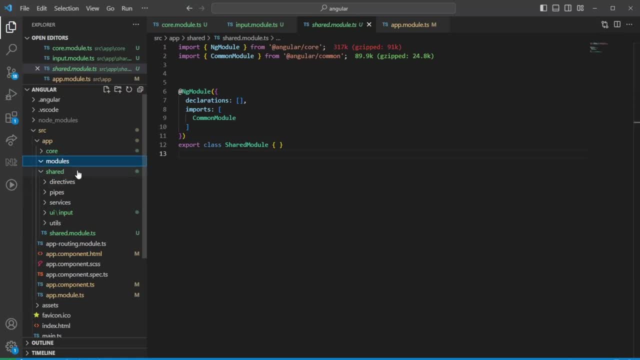 amongst the modules, so something that would be used in more than one module. so now we're going to talk about the module. this is the thing where it might vary a lot between the project. so one thing i would recommend is essentially, let's say we have a module here. in this case, we'll 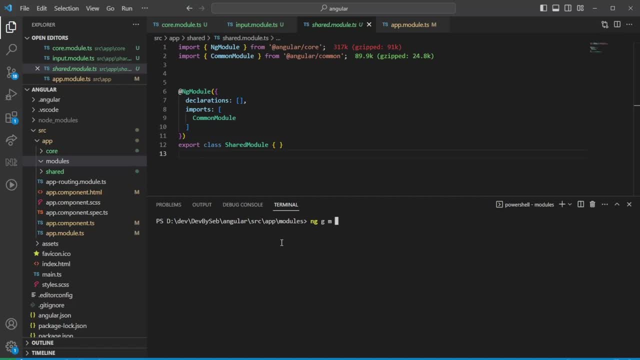 generate a module. let's call it account. so in this case we're going to place everything related to one account within here. it could be a profile page, it could be you name it. it could be anything related to a user in this on your account, it could be yeah, changing your password. it could be all of. 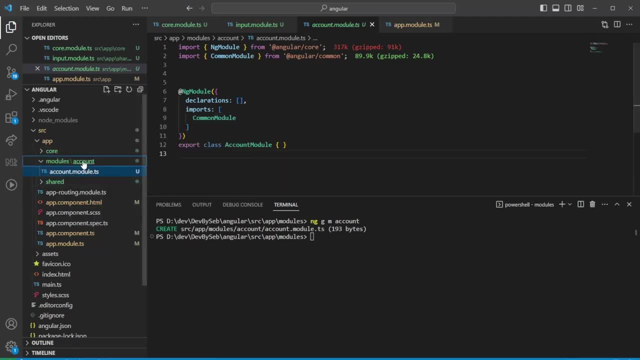 these different stuff that would be placed here. so usually what you do is you generate a module and within the module you would have components and you could have even like for this feature or module you might have services. that's only related to this place. so here's where you should place them and of course, you would have 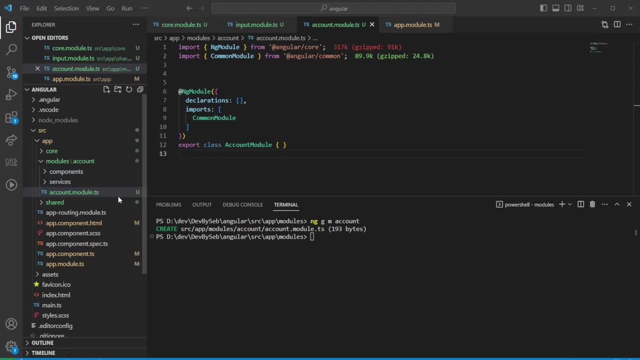 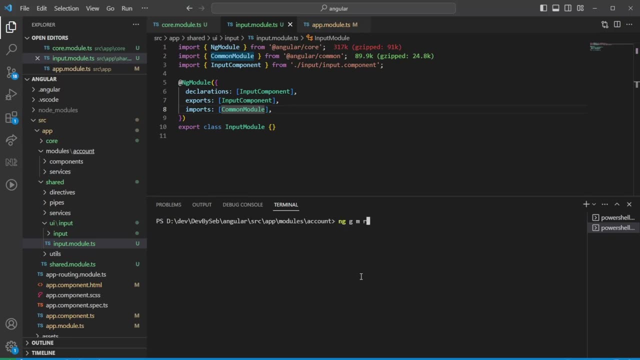 want to have a routing module as well. you, i could have generated that. that was my mistake. so in order for you to generate that, you can say an angular generate module account. i will keep it personal and we'll say routing. so when you, when you hit the routing flag, it will automatically. 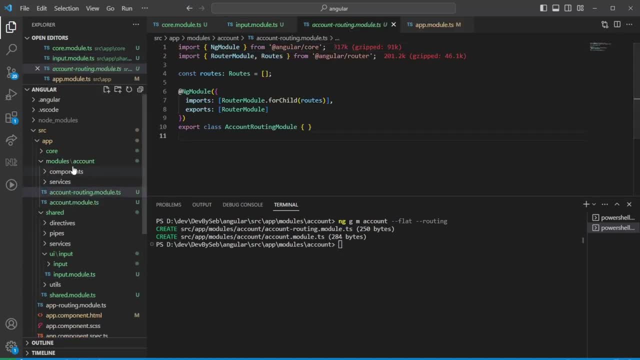 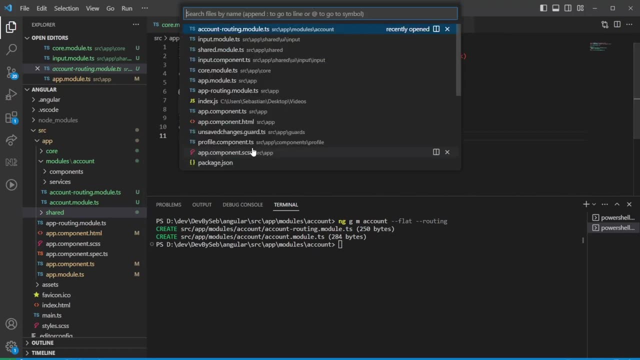 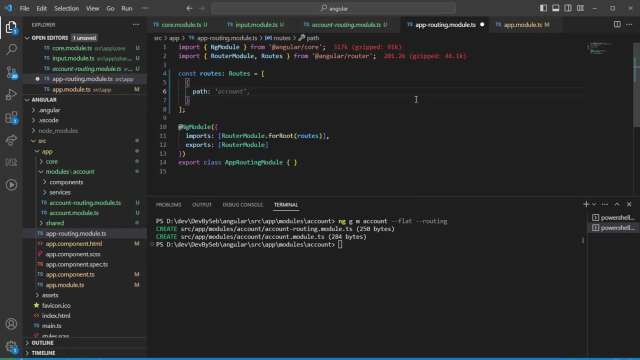 generate a routing module for you. so if you would now, this would enable for you to actually set up lazy loading, which is quite awesome. uh, so if we go to the app routing module, you could just point towards the. so you say, when you hit the account page, we want to load children and in this, 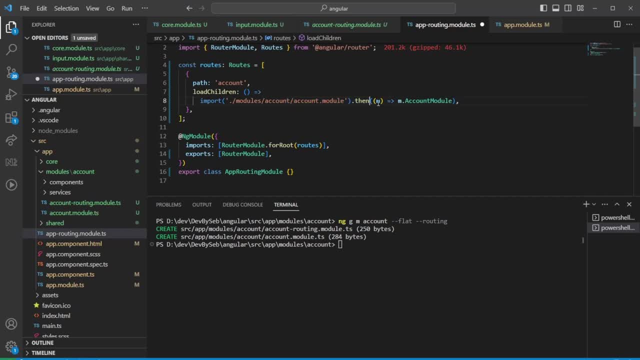 case, we're going to import and whatever comes next. so we're going to load kids and that's where we're actually going to import the students. so in this case, we're going to import and whatever comes next comes from the account module. so now we have set up a lazy loading module which 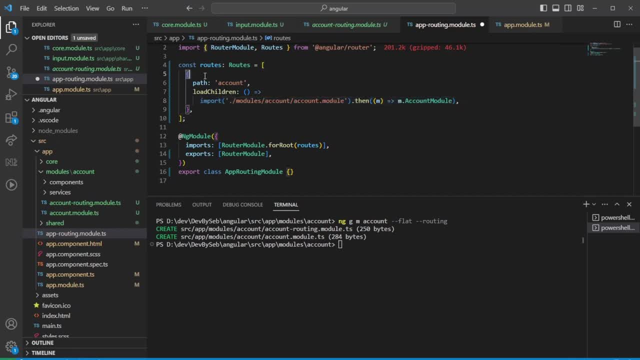 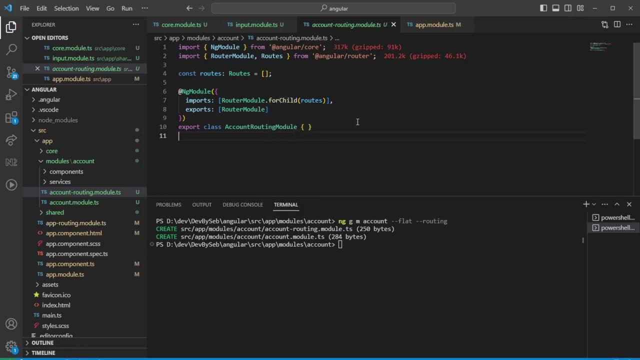 means that we will only load this chunk of code when we hit this path, which is quite awesome. so this is one way. I have another video about lazy loading modules. please feel free to look at that if that would be of interest. so now coming back to this module. so we have the accounts module. it has its own components. it has 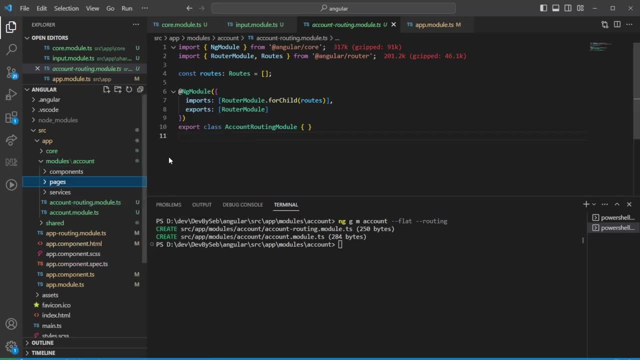 its own services and in many cases, I would also recommend putting pages. so if you want to distinguish which components are visible components versus what components are used within the visual parts or the pages per se, I would recommend having this structure. becomes much easier for you to work with because 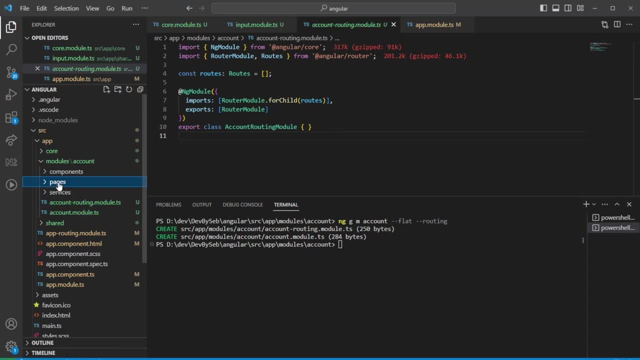 you will automatically understand. okay, whatever is within the pages is what we have set up in the route, so you wouldn't have to go the other way around looking here and checking which components is being used as the pages and whatnot. so this is what I would recommend: setting up a structure like this. it would simply. 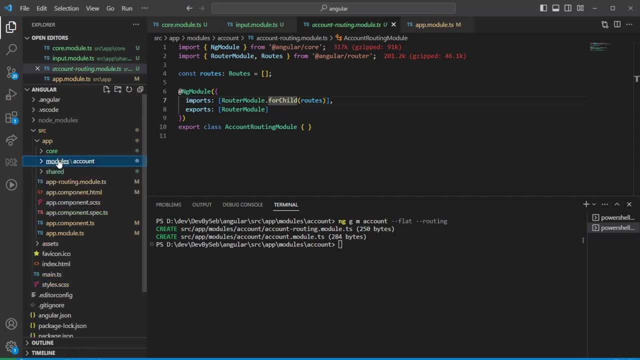 simplify a lot when it comes to working in this way. so this, my friends, is a recommendation on how to work with it. there is no significant way or no exact way without understanding the business logic. also, keep in mind that if you don't have any peer dependencies from the modules to between the 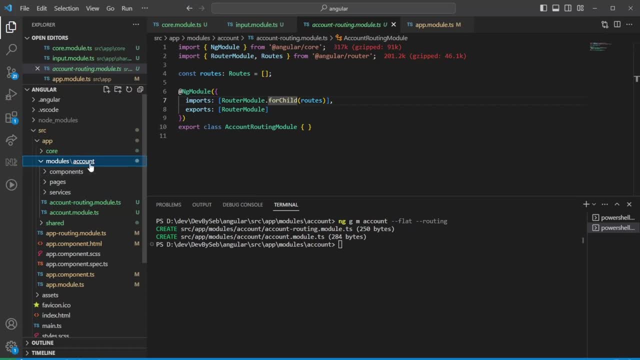 different modules. it might be easy to break it out later, to maybe start working with micro for intense and so on. so now, one thing I want to recommend is that if I, let's say, I want to use the input module in the accounts module that we generated, I would just have to import the input module in this way and if you, 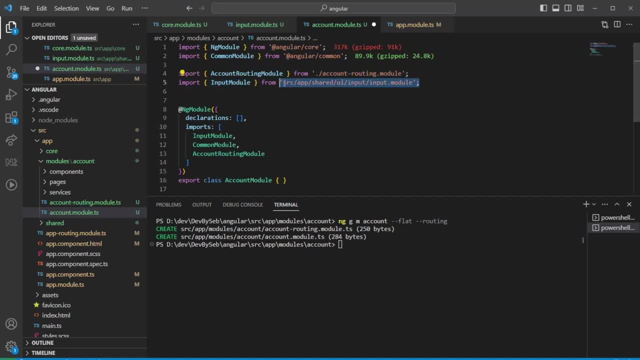 just take a look at this: the, the import source. it looks like it's it's. it's so ugly. so there's a couple of ways we could improve this. we could do it by, first and foremost, working a bit with the TS config file to make sure we have alias to set up so that it looks. 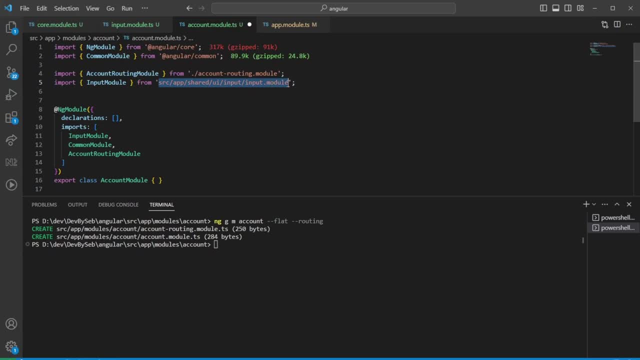 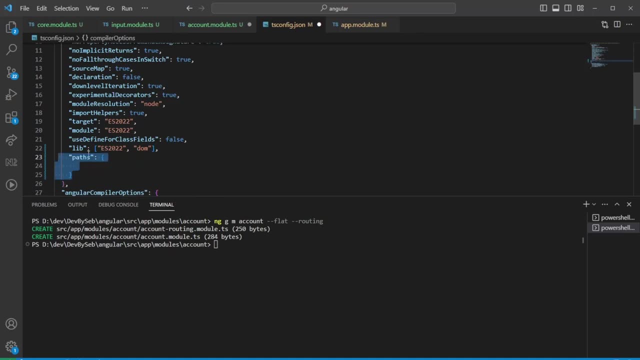 nicer. so the way we could make this even better would be to jump into the TS config file. here we could go ahead and add some paths within the compiler options and we say, whenever we use this alias, we want to point it towards this source. so, uh, UI slash, anything would be matching whatever we have there afterwards. so if 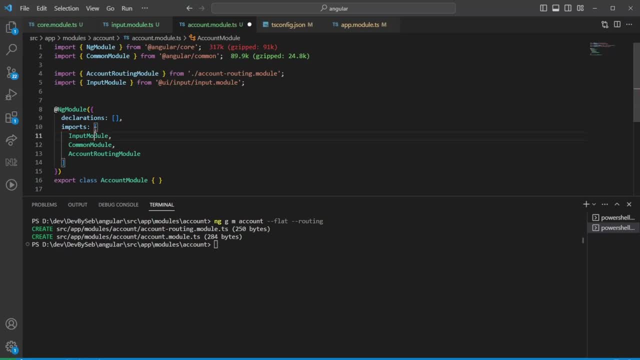 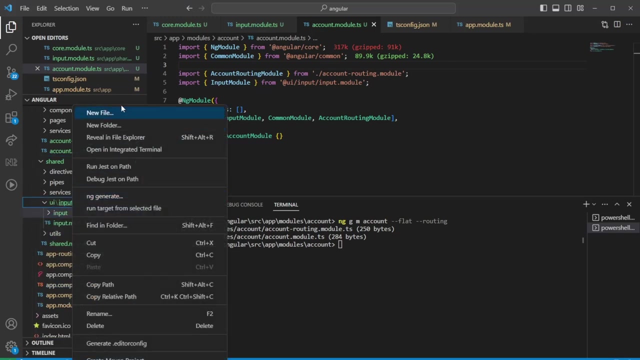 you look here now we should be able to to import it from UI slash input, slash input module, which is also not very nice. so we could now start working with something called barrel functions or about sorry barrel files really. so in this case we would go with within the input, would have an inputts file which 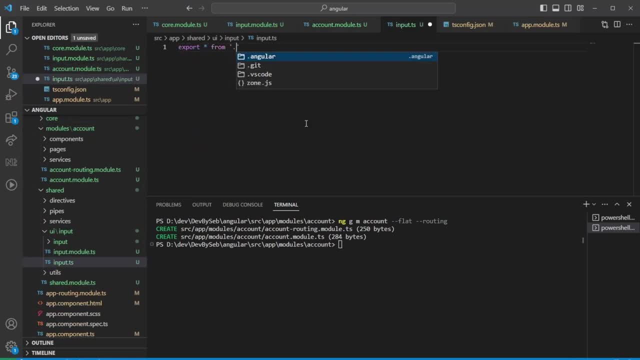 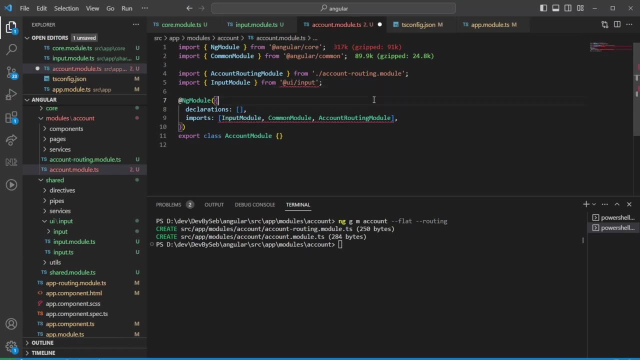 essentially would just export uh star from input module. so if we now look at it, we should be able to import it from, should be able to import it through the input slash input, which is also not very nice. there's also even better ways to doing it. we could also have another. 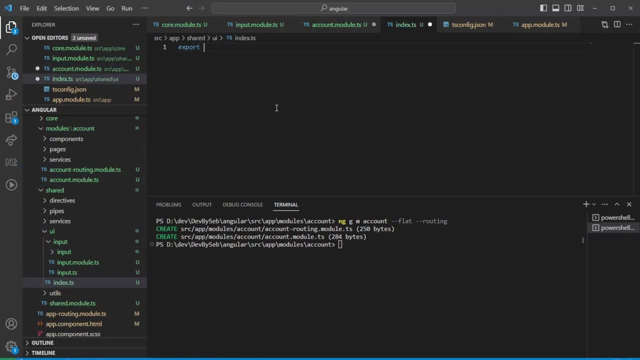 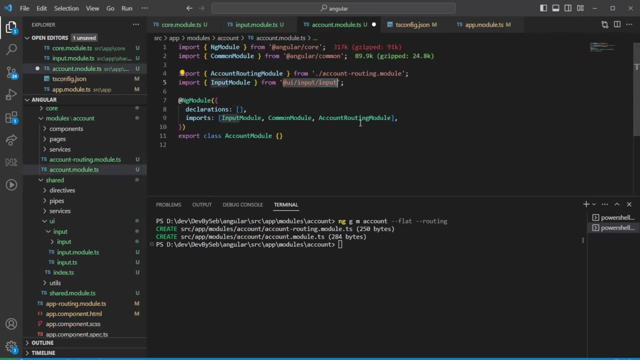 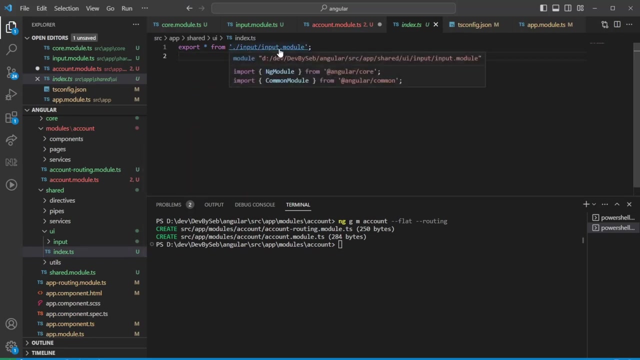 outer index TS file. so here we would just export anything that comes from the input input module module. so in this case we should be able to just import it from the UI if everything is set up correctly, which it seems not to be, because we are not importing it from the input slash input like this, and now it should be possible. 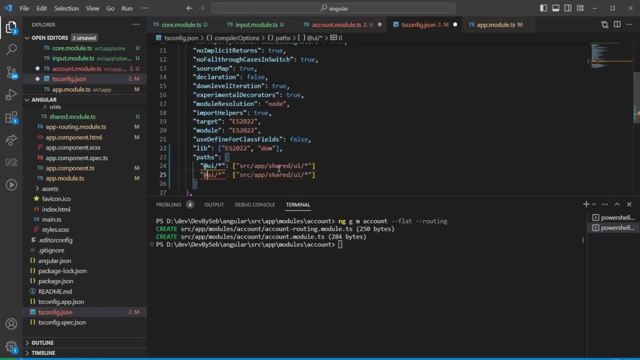 for us to utilize it from there, and of course it won't work if we don't set up the route correctly so we can say: whenever you are on UI, then we are going to prefix with this. so now, when we added the barrel file, we have a file called 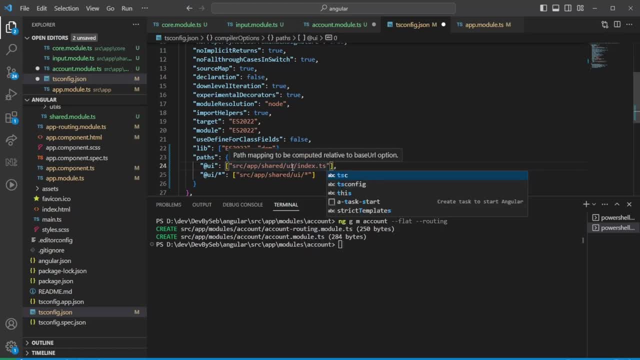 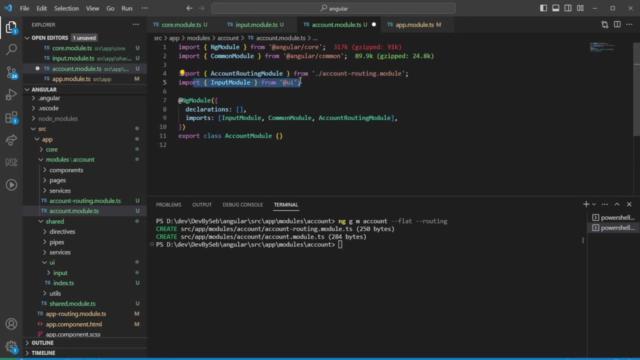 like indexts, which exports the, the input component. but if I now remove this it will be the same thing because it goes towards the indexts file. so now you can see I've imported the input module just from the UI and there you can specify what aliases you want to have for your application, which is super. 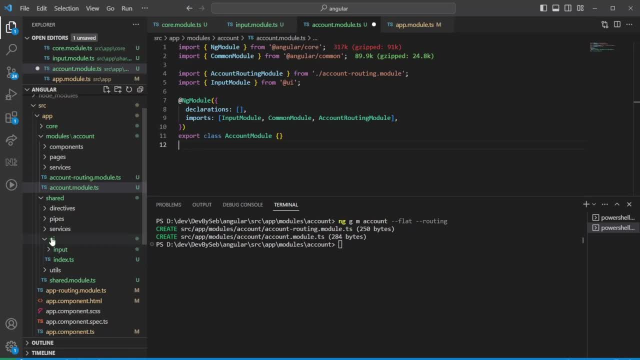 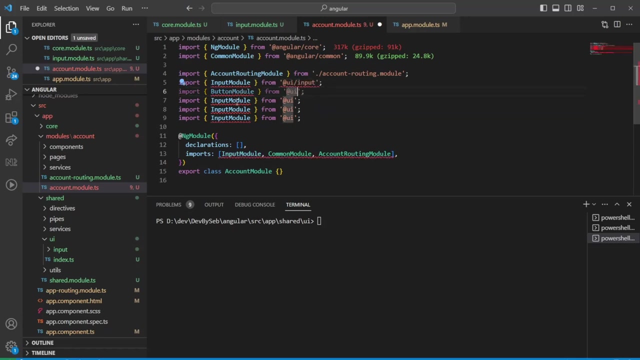 nice. so now imagine, I want to create another component in this UI component library that we have, because we don't want to have multiple import statements. so, for instance, the input would come from slash input and the the button would come from slash button. we could have it in this way, but there's no, no need to do it. 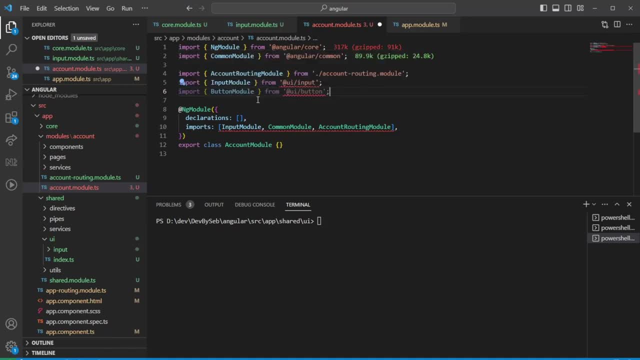 because this is where the bundle optimization will essentially remove stuff that we don't use from us. so what we would want to achieve now in this way would be to add, for instance, a button module which essentially would now come from the same import statement would, which would simplify the code. it would look much better, it would be easy when we